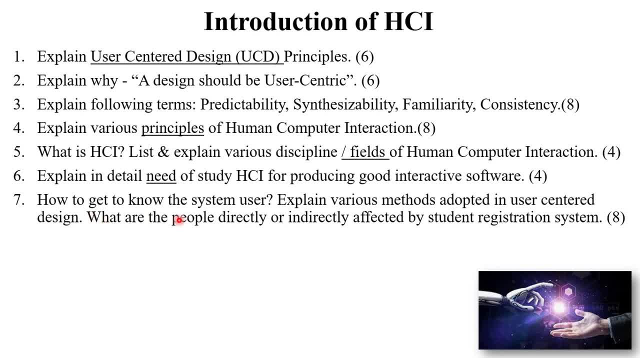 multiple scenario based question. The first scenario is this: how to get to know the system user, explain various methods adopted in user centered design and what are the people directly or indirectly interested in the system. The next question is: what is the need of study HCI or indirectly affected by the student registration system for 8 marks? So you have. 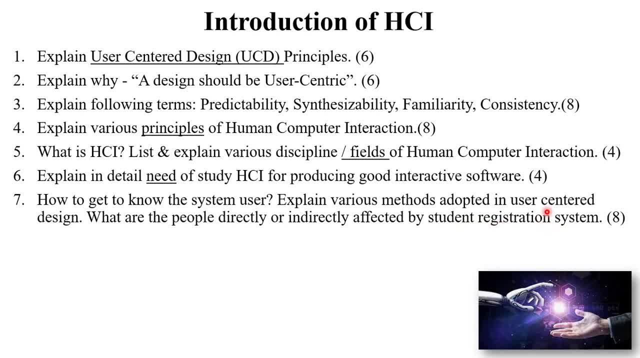 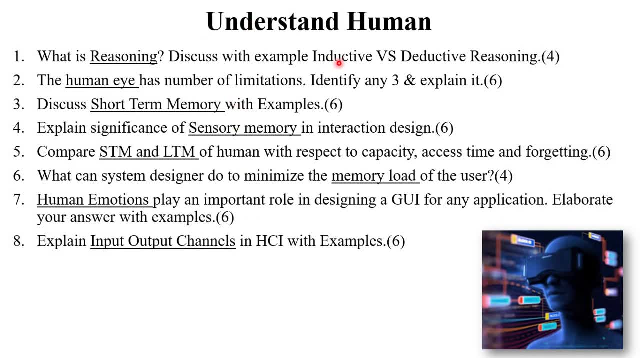 to explain the scenario of student registration system as per the UCD principles. The next on the topic of understanding human. On this topic they will ask: what is reasoning? discuss with example inductive versus deductive reasoning for 4 marks. Here you have to explain. 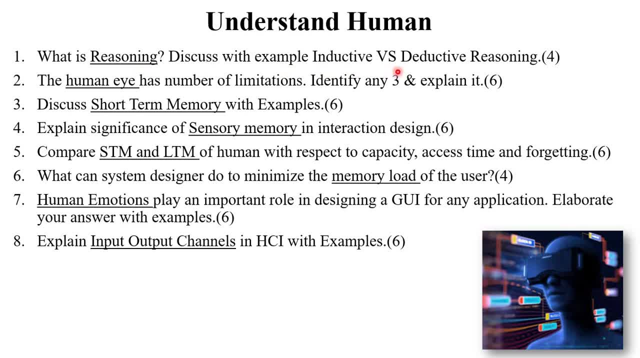 definition of reasoning and explain their types with examples. The next question is: human eye has number of limitations. You have to identify any three and explain it with examples for 6 marks. Next, on the topic of human memory, they will ask any one question from this three question like: discuss short term memory with example. 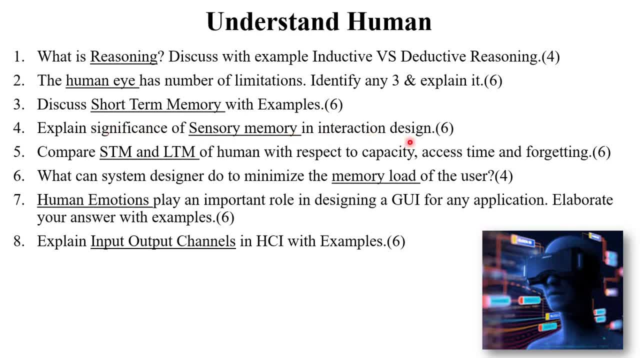 or explain significance of sensory memory in interaction design. or compare short term memory and long term memory of human with respect to capacity, access time and forgetting. So this three question generally asked for 6 marks. The next question: what can system designer do to minimize the memory load of the user? for the 4 marks. The next question on the 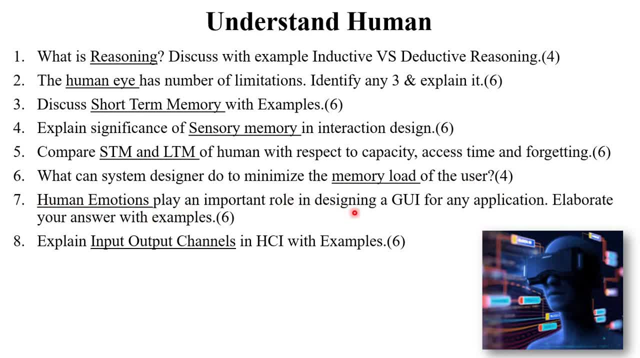 basis of human emotions. like, human emotions play important role in designing a GUI for any application, So you need to elaborate how human emotions will be helpful for designing, with examples for 6 marks. The next question is: explain input output channels in HCI with examples. 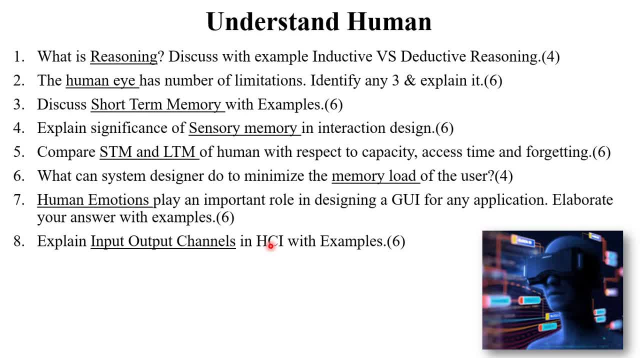 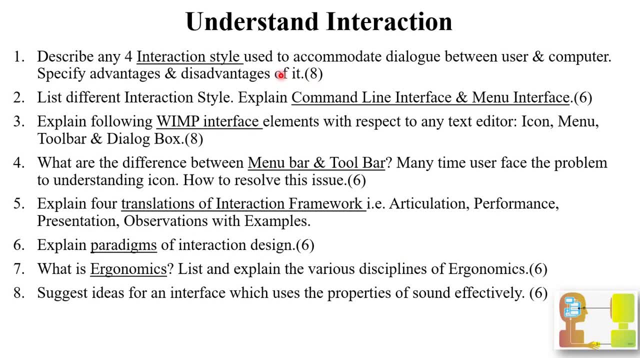 Here you have to explain 5 input output channels, with diagrams and with their examples, point wise for 6 marks. Next, the next most important topic is understanding interaction. On this topic, multiple questions will be asked. The first question either they will ask: describe any four interaction style that used to accommodate dialogue between user and computer and mention 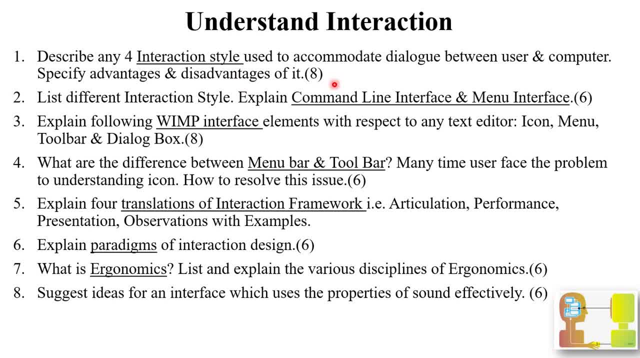 this advantages and disadvantages for 8 marks. Or they will ask list different interaction style and explain specific like command line interface or menu interface. So you have to prepare all interaction style. either you have to explain specific one or you have to explain all the one right for 8 or 6 marks. The next: 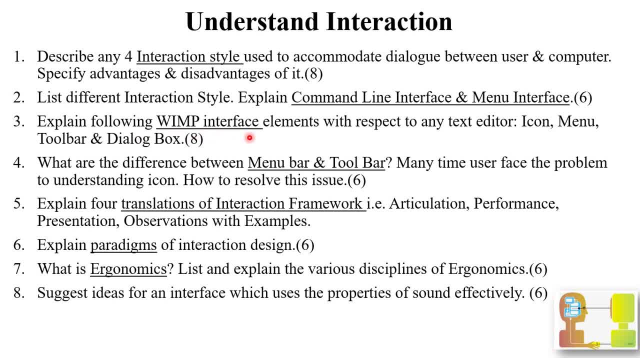 question: most important question, like explain following W IMP interface element with respect to any text editor, like icon, menu, toolbar and dialogue box for 8 marks. The next question Is: this question is the most important question, like explain following W IMP interface element with respect to any text editor, like icon, menu, toolbar and dialogue box for 8 marks. The next question: 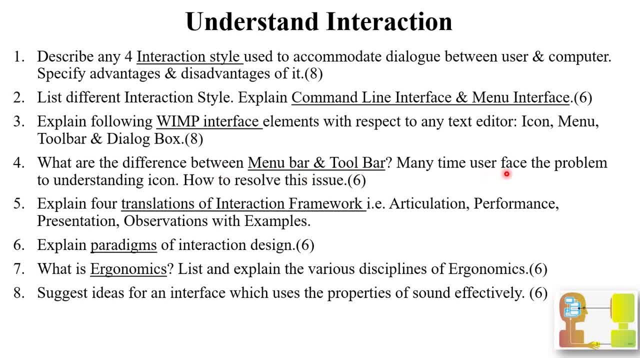 is: what are the difference between menu bar and toolbar? many time user face the problem to understanding the icon between them and how to resolve this issue for 6 marks. So here you have to explain this thing with your own language, with examples, with diagrams. The next question is: explain for translation of interaction framework, that is, articulation. 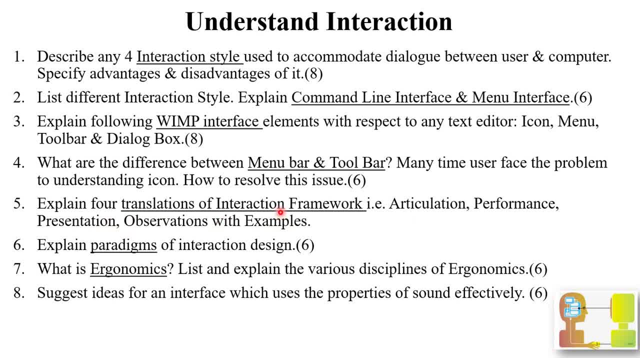 performance presentation observation with example. Here you have to draw the diagram of interaction framework. Here you have to draw the diagram of interaction framework. You have to explain what is the proper naming convention and after that explain this for translations with example, point wise, for eight marks. Next question is: explain paradigms. 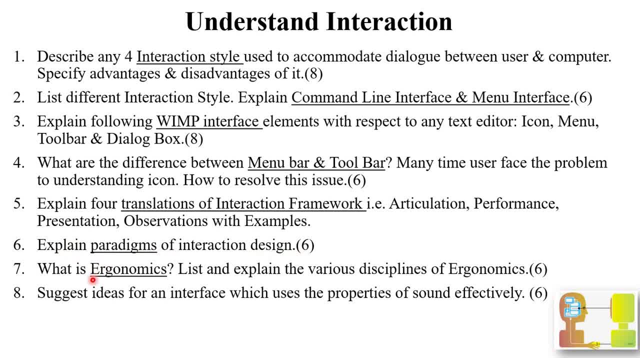 of interaction design for six marks. and again, most important question: what is economics? list and explain various disciplines of economics? here you have to draw the diagram and list and explain all these economics with examples for six marks. The next question is that is scenario based question, Suggest idea for an interaction framework? Here you have to. 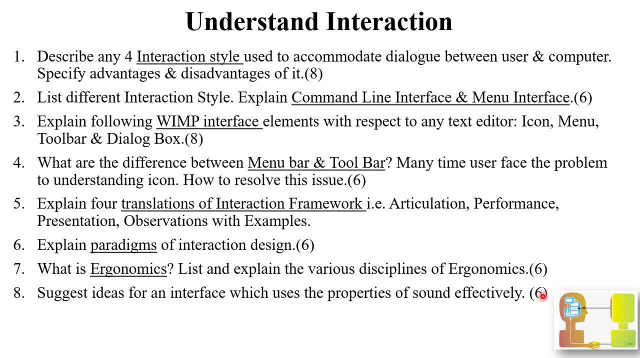 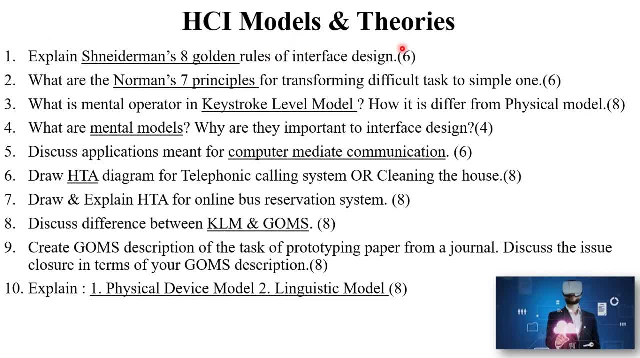 interface which uses the properties of sound effectively, for six marks next. the next important topic is SCI models and theories on the basis of this topic. they will ask: explain Snyderman's eight golden rules of interface design. here you have to prepare all the golden rules, proper naming conventions and explain this with examples. for six marks next, what are the Norman seven? 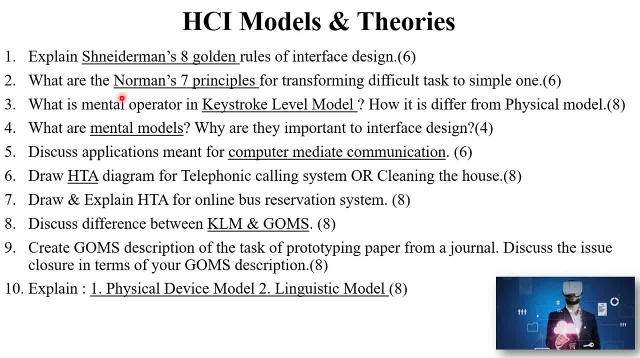 principles for transforming difficult task to simple one. here you have to mention all the Norman seven principles, with explanation point wise, for six marks. the next question is: what is mean by keystroke level model and how it is different from physical model? for eight marks. next question: what are the mental model and why are they important to interface? 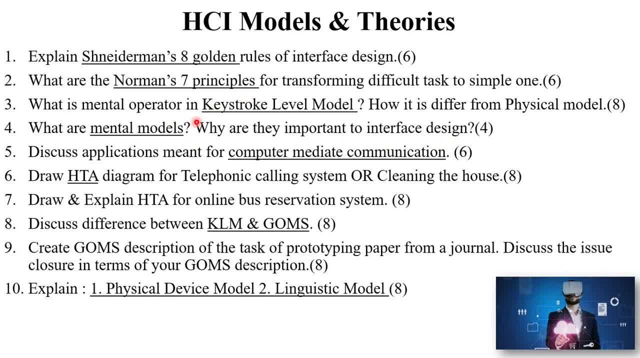 the design for four marks. so here you have to draw the diagram of this model and explain point wise. Then the application meant for computer mediated communication, for six marks. the next important topic is HTA, right. so here you need to draw HTA for any particular application that will. 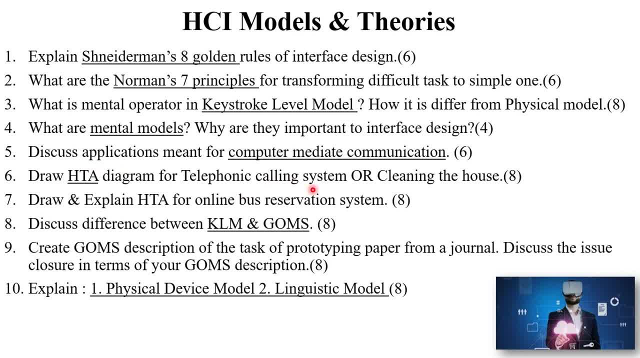 they will ask in your exam, like HTA diagram of telephonic calling system, HTA diagram of cleaning the house or HTA diagram of online bus reservation system, you have to prepare specific HTA diagram and their explanation for eight marks. this is a compulsory question. 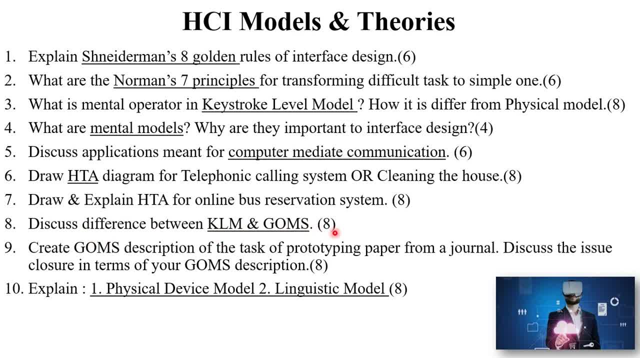 the next one is: You have to discuss difference between KLM and GOMS model for eight marks. you have to mention any seven to eight points regarding this model. the next question is scenario based question like create GOMS. description of the task of prototyping paper from journal discuss. 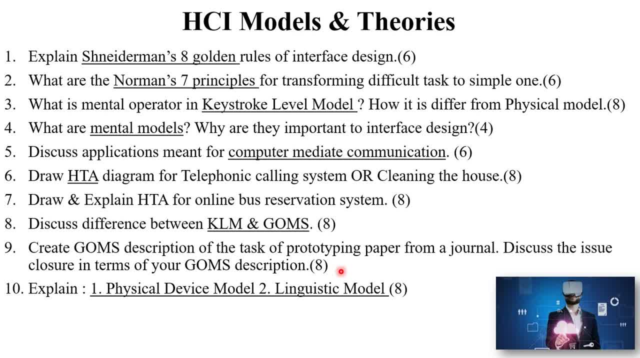 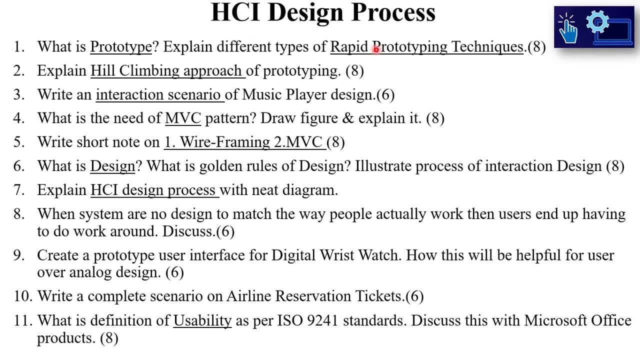 the issue closer in terms of GOMS description for eight marks. and last question is: you have to explain this. two models for eight marks, like physical device model, linguistic model- here You have to draw the diagram, You have to discuss their explanation. The next important point is HCI design process. on this topic they will ask most important. 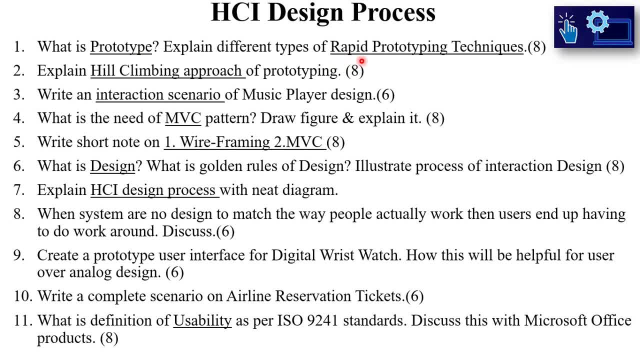 question. that is first question: what is prototype? explain different types of rapid prototyping technique. here you have to mention the definition, their types, with example and with proper point wise explanation for eight marks. the next one is explain hill climbing- approach of prototyping for eight marks. 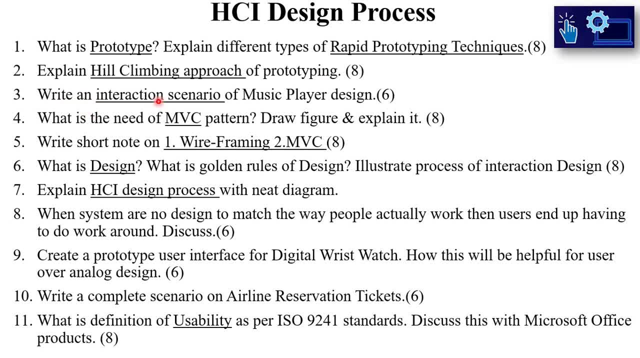 Then there is a scenario. I will give you the test question it is, and then we will keep review those next three key areas which are demonstration of these processes. then you can, dad, describe these- and this is the best question, right- and interaction scenario. 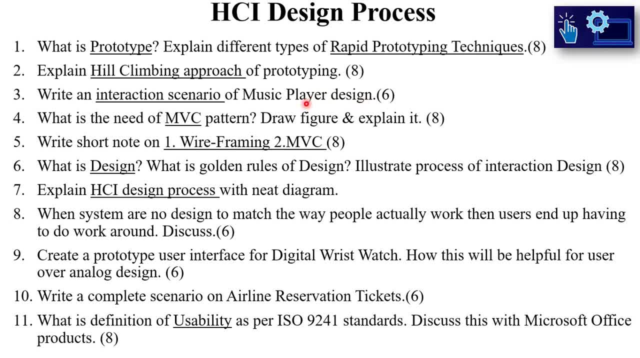 of music player design means how music player design will be developed, how user use this music player design, these types of functionalities there. you have to explain this thing in your own language for six marks. the next important point is mvc and wireframing. so they will ask any one question like: what is the need of and VC pattern draw, figure an. 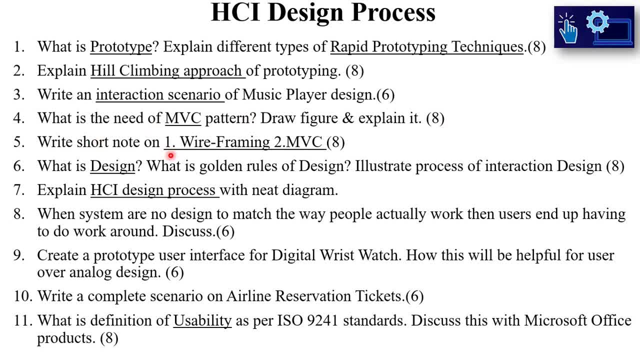 explain it for eight months. or they will ask: write a short note on wirefram or and VSE for eight month. The next important point: mvc and wireframing. So they will ask any one question like what is the need of mvc pattern, draw figure an. explain it for eight months, or they will ask: write a short. 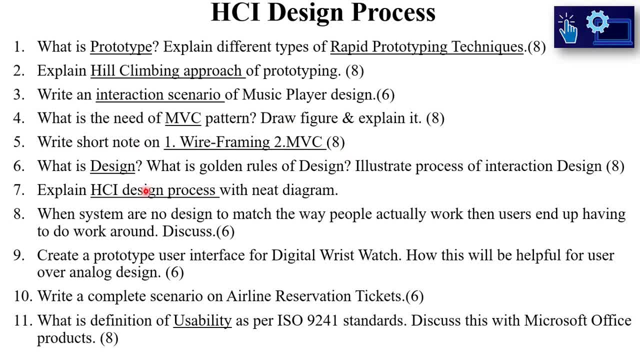 note on wire framing or MVC for 8 marks. the next they will ask any one question from this: what is design, what is the golden rules of design? and you need to illustrate the process of interaction design for 8 marks. or they will ask: explain HCI design process with knit. 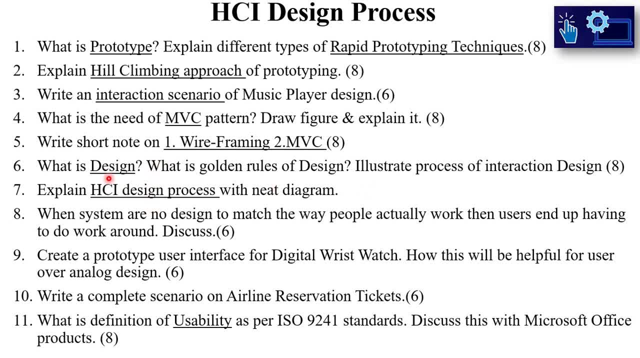 diagram for 8 marks. so you have to explain their definition, their golden rules, their diagram of HCI design process with proper explanation. the next, this remaining four are the scenario based question, like when system are not designed properly to match the way people actually work, then how user end up having to do the work. so you need to 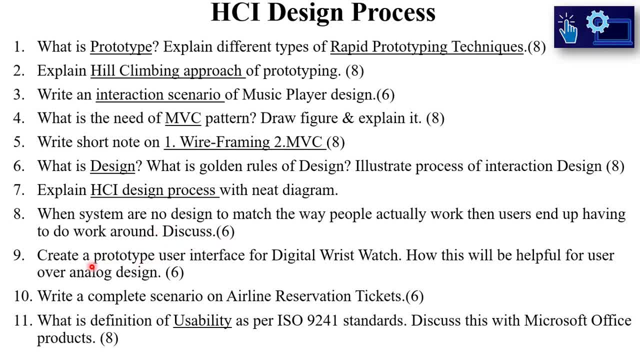 discuss this thing for 6 marks. next scenario based question is: create a prototype user interface for digital wristwatch. suppose there is a prototype of digital wristwatch, so how this prototype will be helpful for user over analog design for 6 marks. and next scenario based question is write a complete 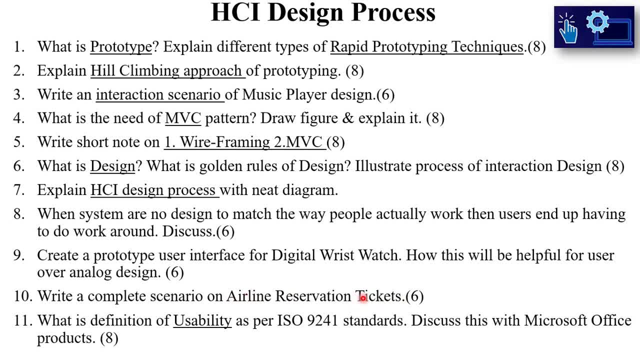 scenario on air rail reservation tickets, so how this particular applications have made and how which type of functionalities they will provide. so you have to explain any one scenario with 6 marks in your own language, point wise, with examples. and last question is: what is the definition of usability as per ISO standard? so you have to mention the 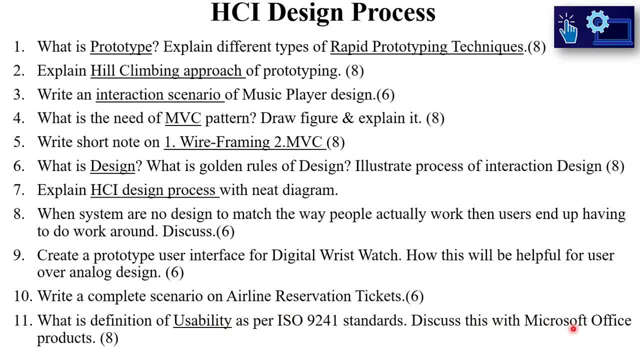 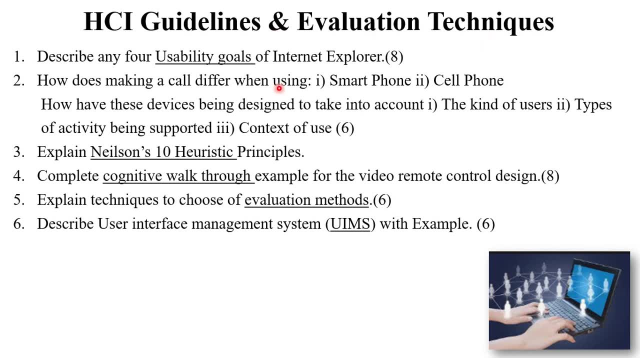 definition usability and how this definition will be helpful with Microsoft Office products means Microsoft Office products. how provide the different usability techniques for 8 marks? the next topic is HCI guidelines and evaluation technique. on this topic they will ask the first important question: describe any four usability goals for internet explorer. so generally, on this, 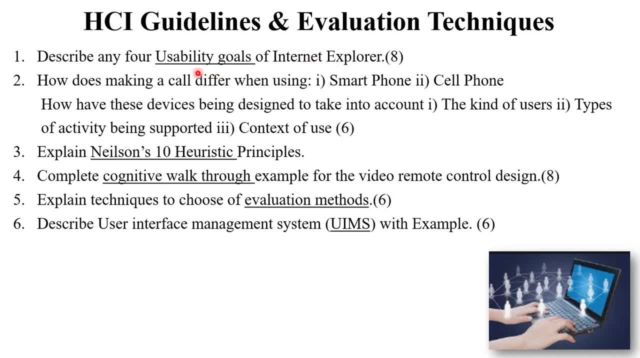 topic. they will ask scenario based question: how internet explorer usable for the user for 8 marks. the next one is: there is a smartphone and cell phone. so how it is different, how it is usable to the user for 6 marks. then explain nelson's 10. 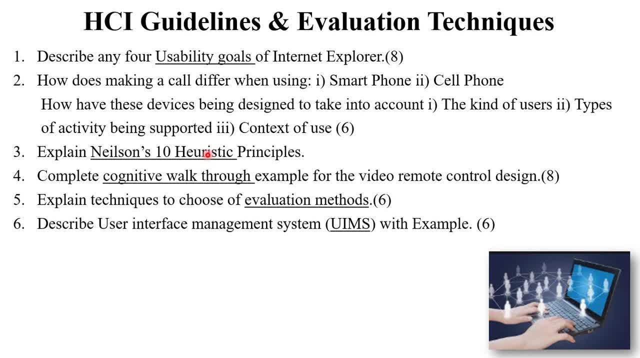 heroistic principles for 8 marks. this is one of the most important question. then complete cognitive walkthrough example for the video remote control design for 8 marks. this is also most important topic: cognitive walkthrough design. you have to prepare this. the next one is explain techniques to choose evaluation method for 6 marks and describe user interface management system with.